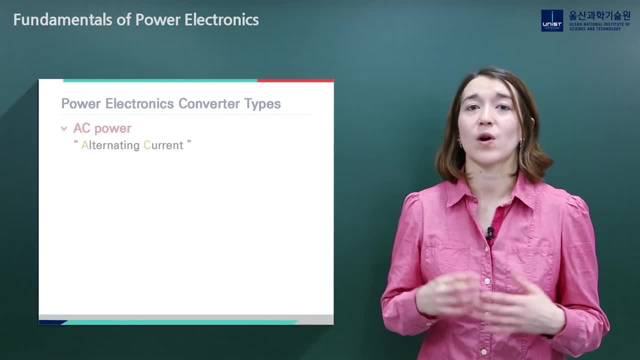 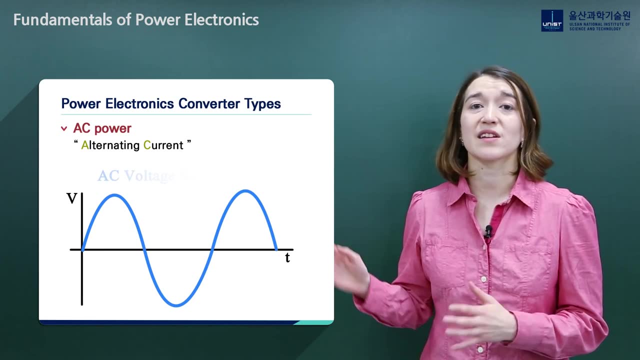 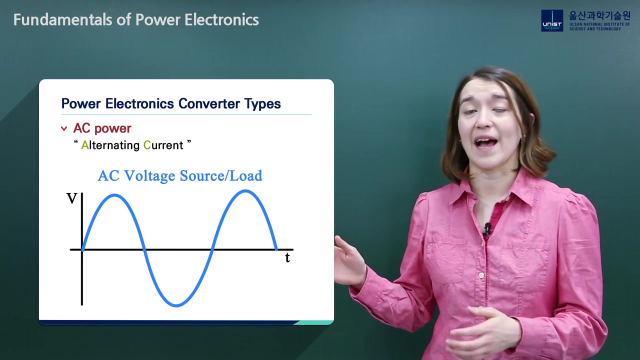 The second type is called AC power. AC stands for alternating current. Again, we think about it in terms of voltage, And here you can see, over time the voltage is actually going to change: Starts at zero, but then becomes positive and then goes back and becomes negative as time. 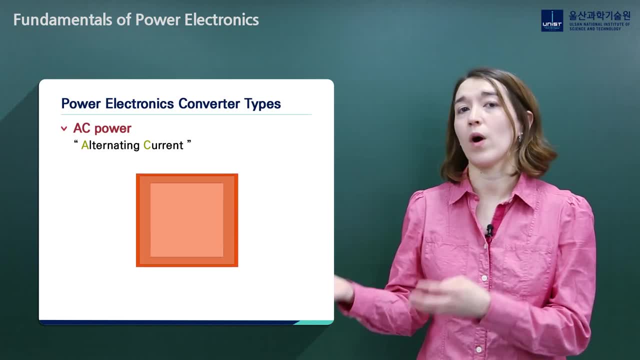 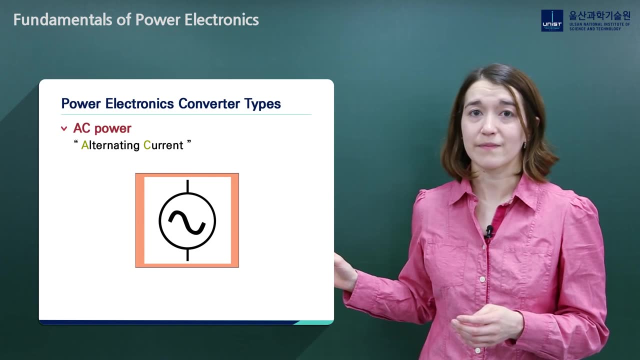 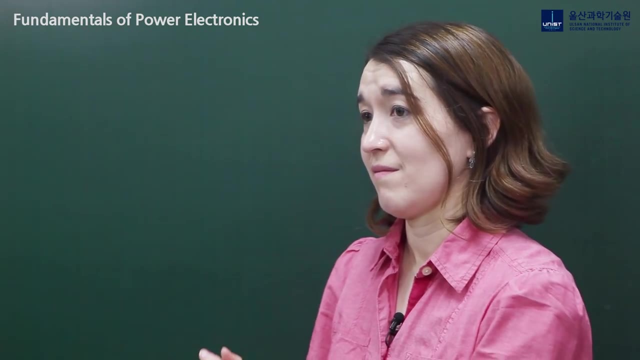 passes. An example of this is wall power. The power we get from the outlet is an AC power, and so the voltage is changing over time. The symbol for this is shown here as well. Now we want to use power from one source to the load, and we may have to change from one. 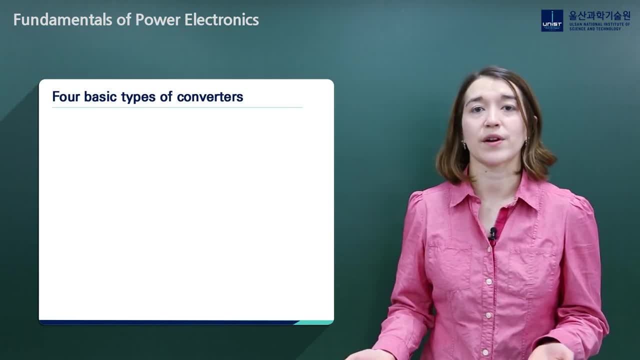 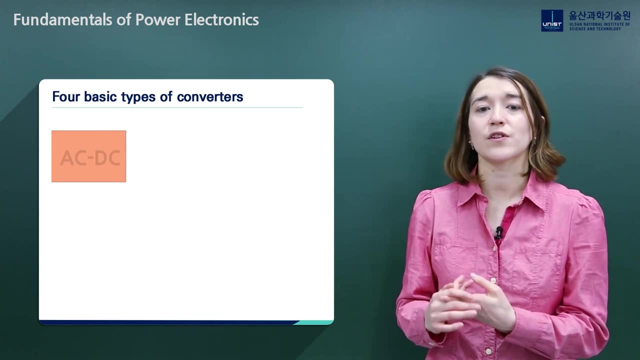 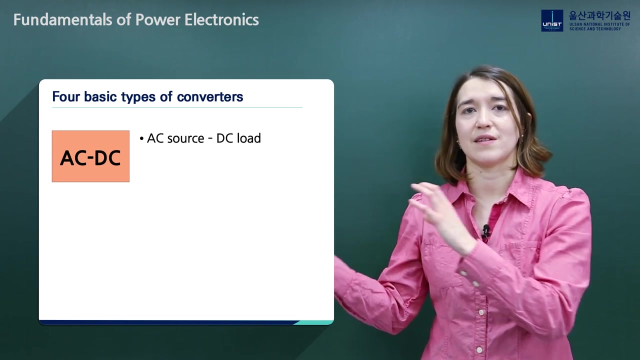 type to the other. So we have to use a power converter to convert from one to the other. There's four basic types of converters based on the power. The first one is AC to DC. So we take a converter and we have an AC source DC load. 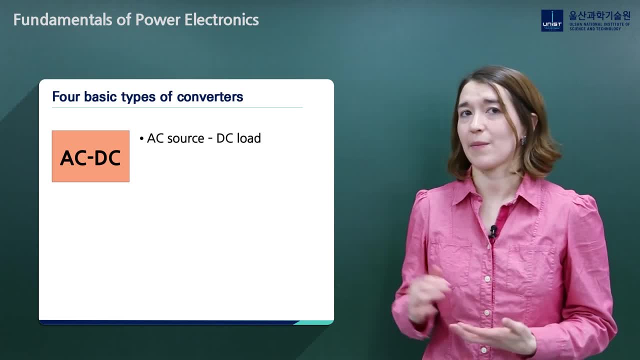 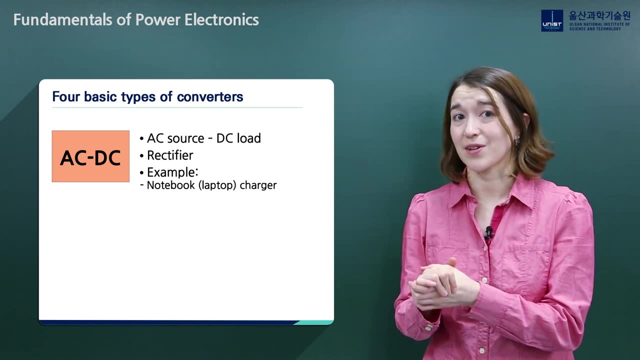 AC to DC. We use an AC-DC converter to change that power. This is also called a rectifier. One example is a notebook charger- laptop charger- where we use the wall power and we change it into DC power to charge a battery. 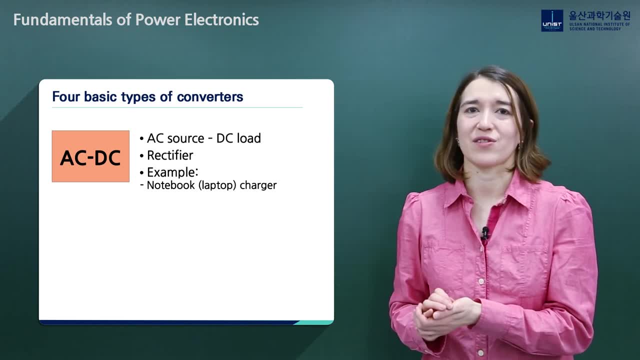 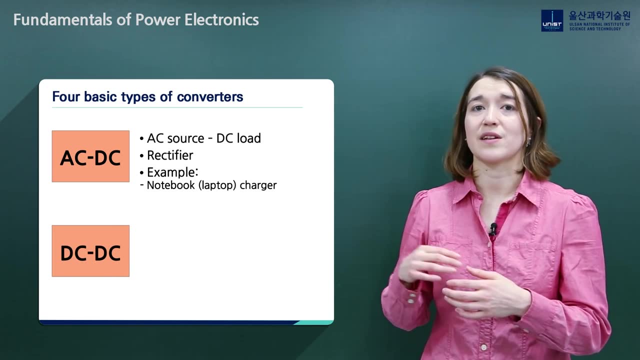 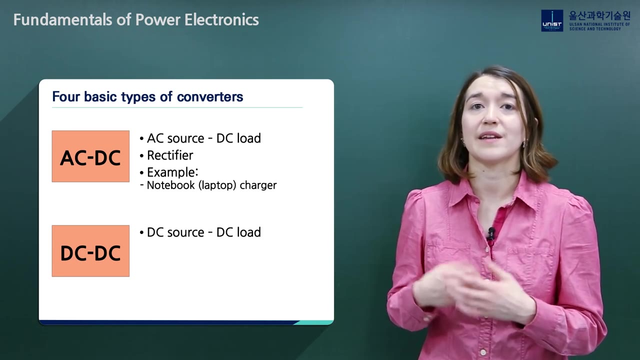 This is an example of a rectifying power electronic circuit. The second one is a DC to DC converter. In this case we want to change, maybe, the voltage of one DC. We want to change the voltage to another voltage, So we can use a DC-DC converter. 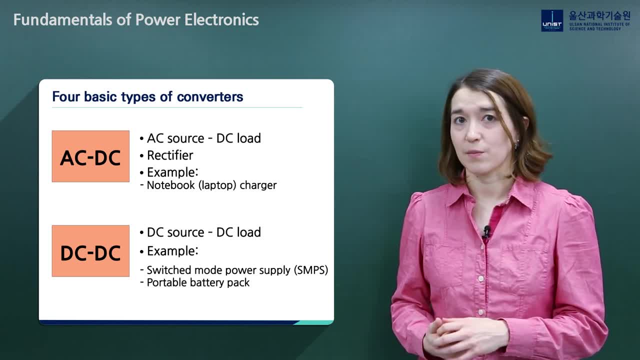 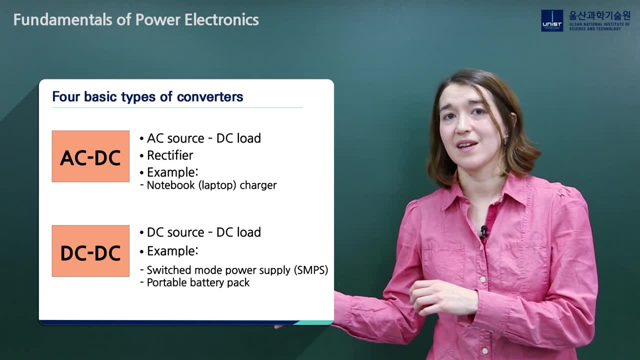 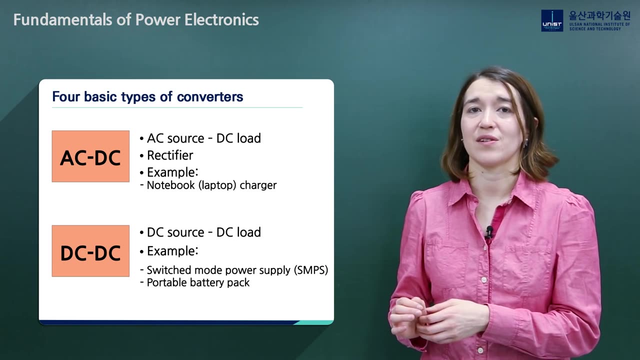 A very common example of this converter is a switched mode power supply. We might see this in a battery charging, So USB to battery charging application like a portable battery pack. We would use a DC-DC converter to do this. The third form would be going from DC power to AC power. 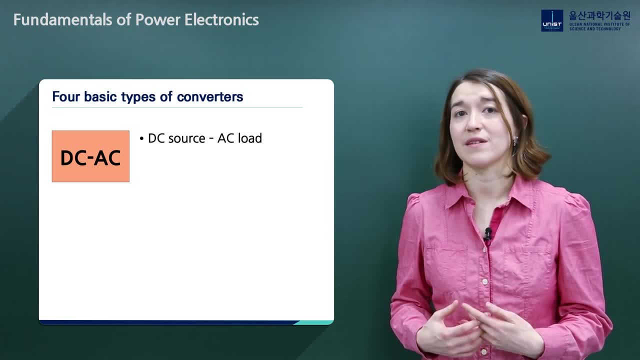 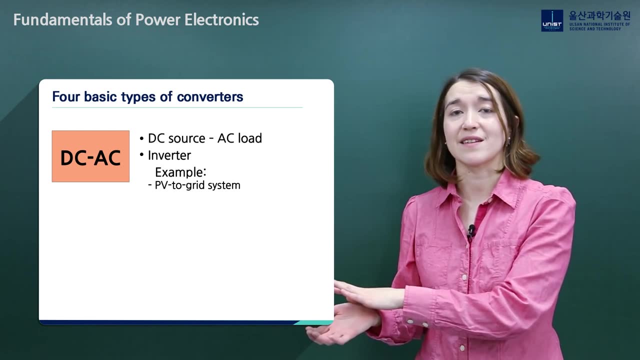 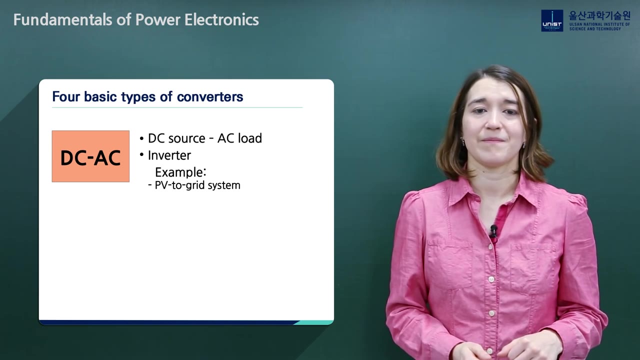 We call this a DC-AC converter. Another common name is an inverter. In this example, you may go from PV power, photovoltaic power, which is DC, to the AC load, which is the wall power. So in this case we'd go DC to AC.